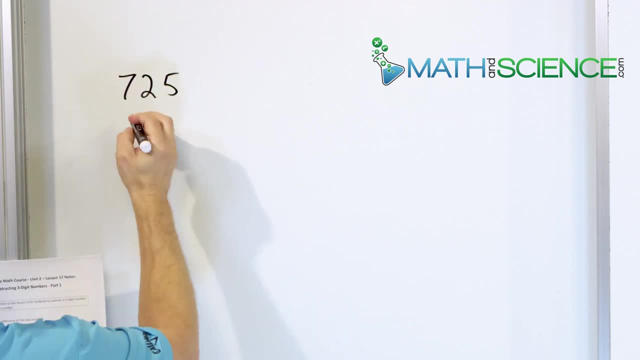 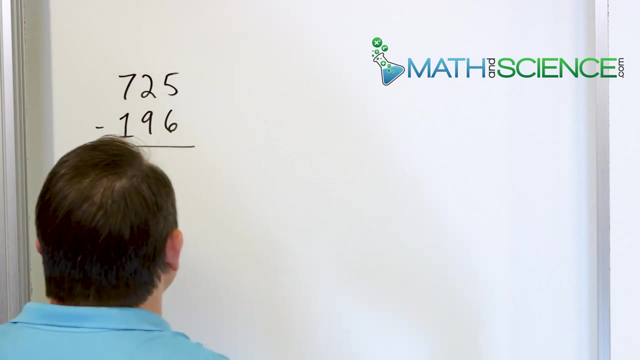 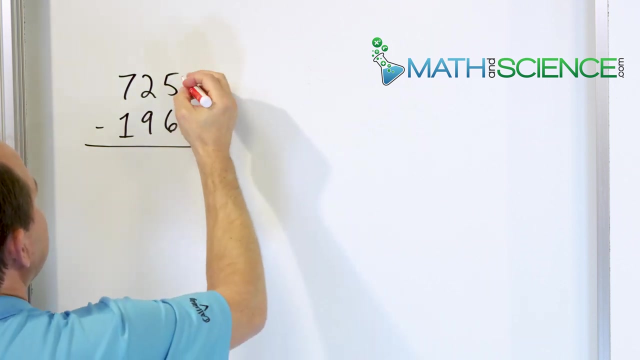 725 and you want to subtract from that 196.. So we draw the minus sign and the bar like this. Now the right hand column says we need to take 5 and subtract 6, but the problem is, 5 is not big enough to take away 6.. So what do we do? We turn that 5 into a 15.. How do we do that? We borrow it. 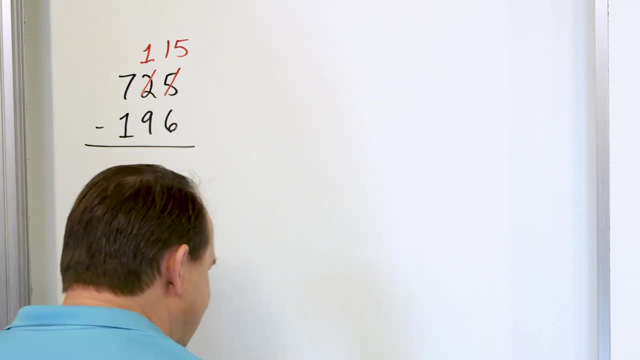 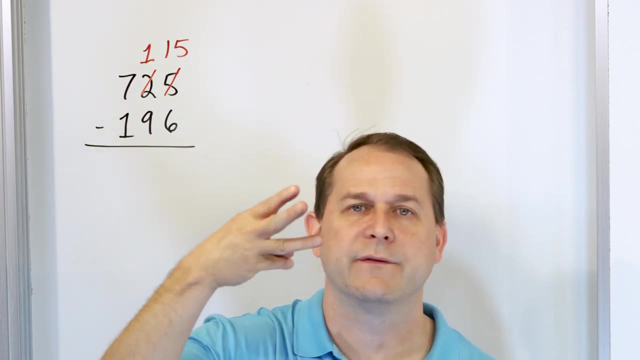 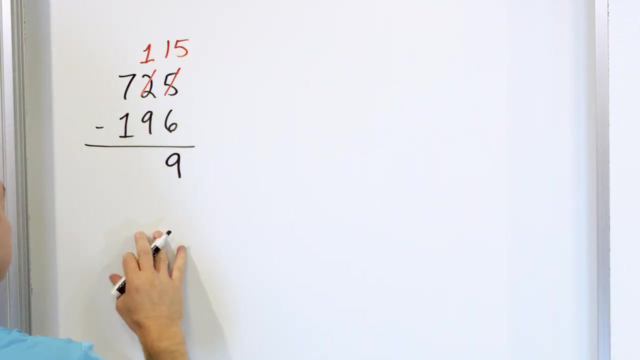 from next door. so the 2 becomes a 1.. So now we can say 15 minus 6.. Start with 15 in your mind and you go down 14,, 13,, 12,, 11,, 10,, 9.. So 15 minus 6 is 9.. All right, Next we go into the. 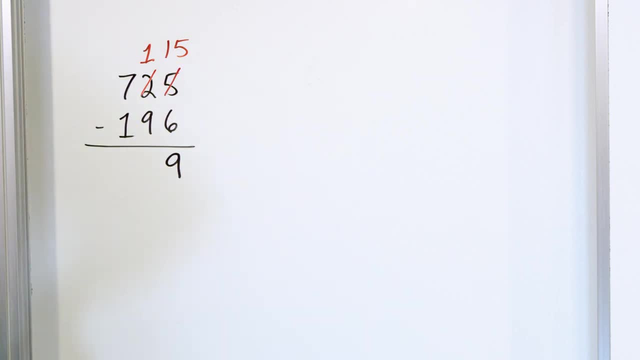 column next door, 1 minus 9.. Same problem: 1 is not large enough, so what we have to do is make this 1 into an 11.. How do we do that? We borrow it from the next door, 7, and make it a 6.. 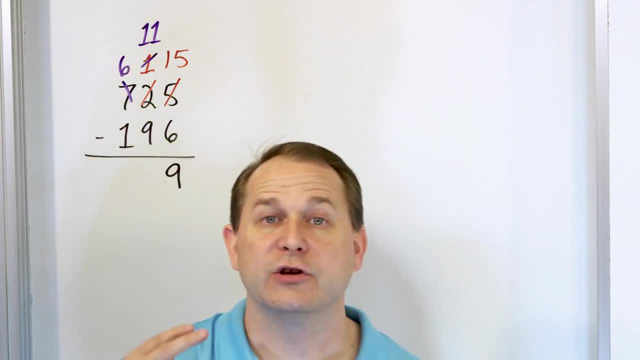 So now we say: what is 11 minus 9?? Start with 11.. Go down 10, 9,, 8,, 7,, 6, 5,, 4,, 3, 2.. So 11 minus 9 is 2, and that goes in this column. Now we go to the third column. 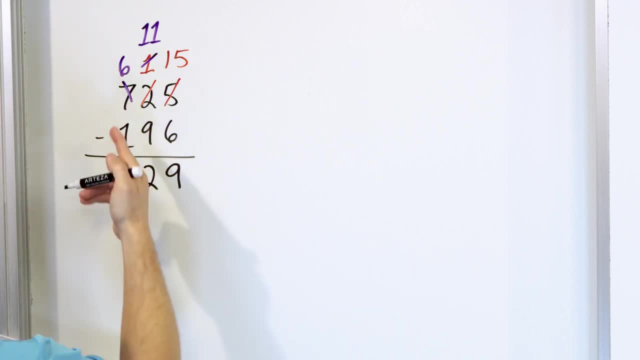 Here the hundreds column here, 6 minus 1, is 5.. You just go down and give it a 5 there, So we have 529.. This is the final answer. Every one of these problems will be done the same way. There are no. 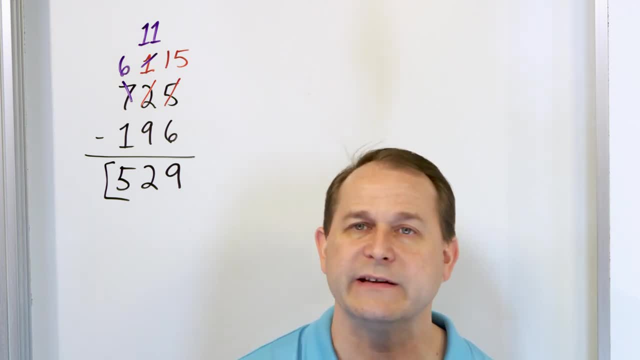 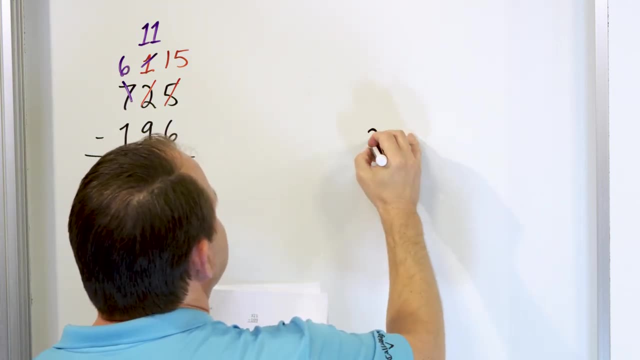 trick questions. Nothing crazy. We're just going to get practice doing the same thing because we have to learn how to do it Very, very easily without worrying about it. Now what if we have 321 and we'll subtract from that 109?? 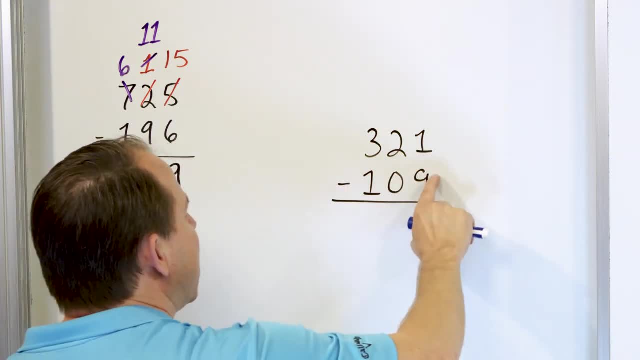 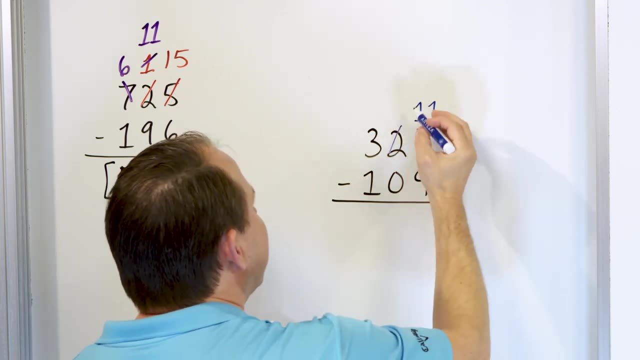 Same thing. Let's go to the right-hand column: 1 minus 9.. Can't do that because 1 is not large enough, So we'll change the 1 and we'll make it 11.. How do we do that? We take it away from the. 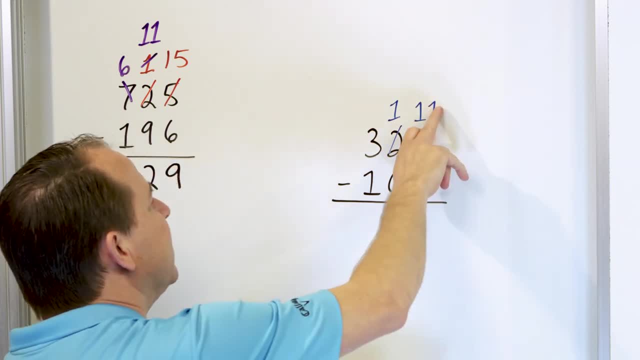 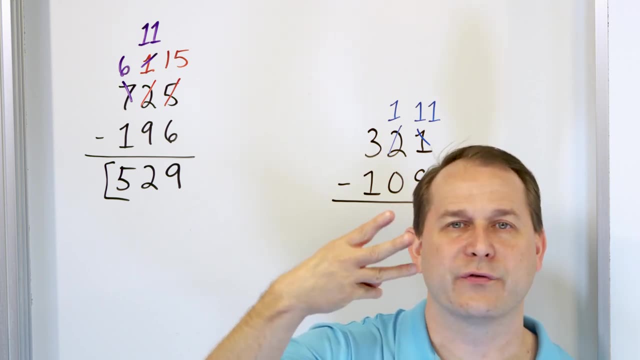 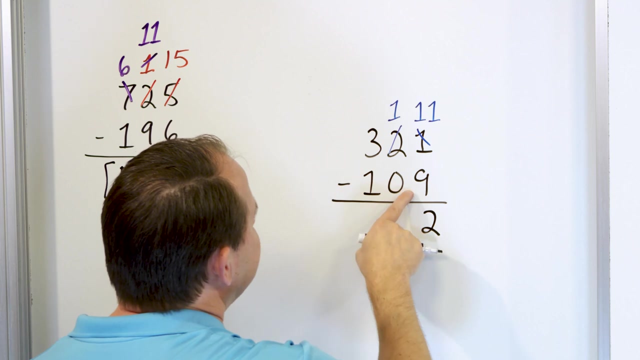 next column. The 2 then becomes a 1.. Now we can say 11 minus 9.. So then we start with 11.. Go down 10, 9,, 8, 7, 6,, 5,, 4,, 3, 2. We land on 2.. So 11 minus 9 is 2.. Now the next column: 1 minus 0. 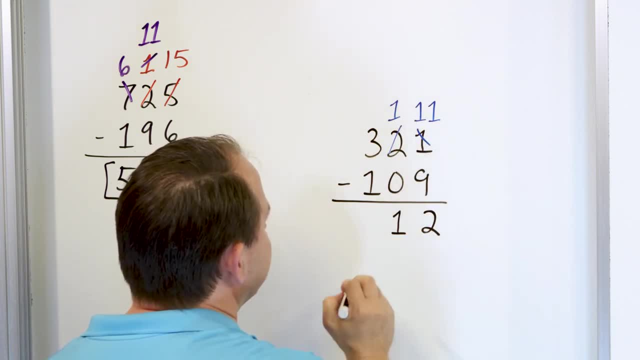 It means we start at 1.. We don't take away anything, so we still have a 1.. Now we go to the next column, 3 minus 1.. Start with 3.. You go down by 1 and you land on the number 2.. So the 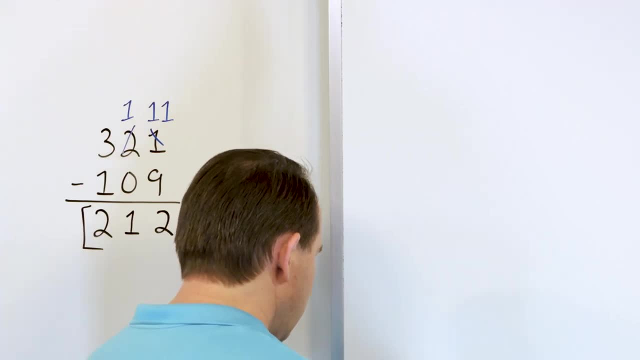 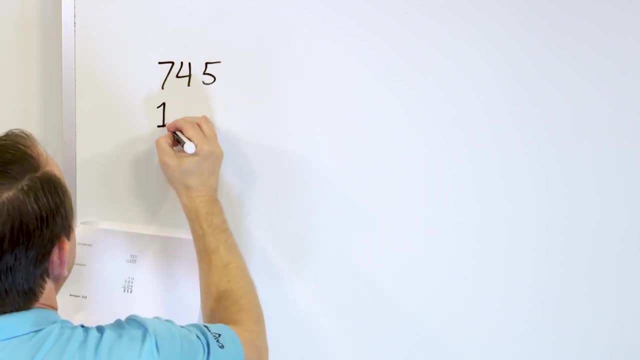 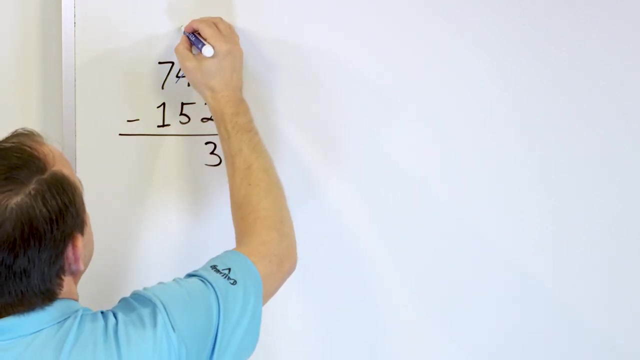 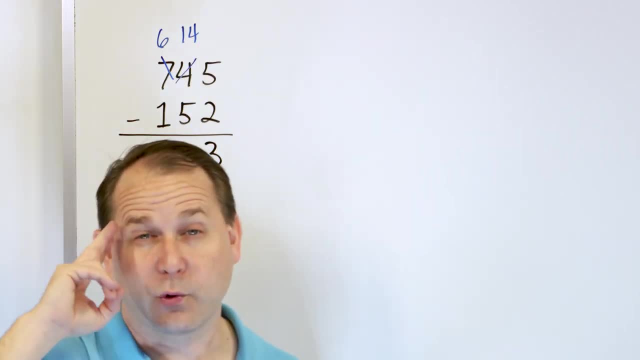 Now what does 14 minus 5? Start with 14 and go down 13,, 12,, 11,, 10,, 9.. And we land on 9.. 14 minus 5 is 9, so the 9 goes right here. Now, in the next column, 6 minus 1 means we just go down from 6. 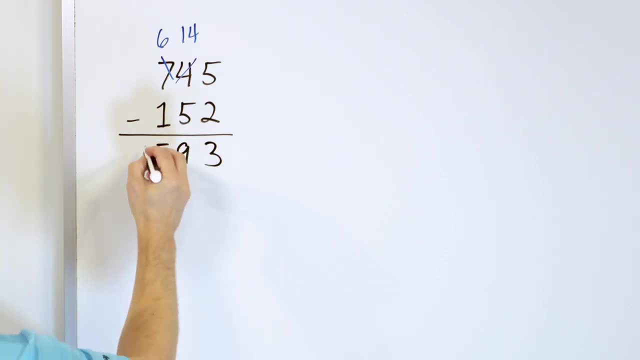 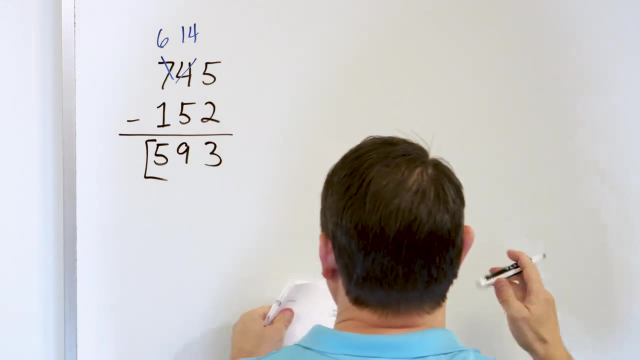 and turn that into a 5.. 6 minus 1 is 5, and we have 593.. That's the final answer. All right, so same process. We're just going to get more practice as we move along here. What if? 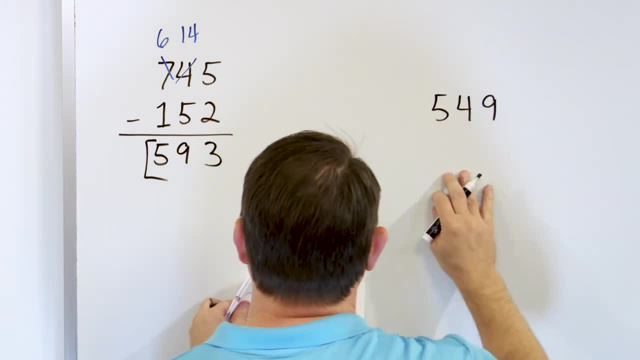 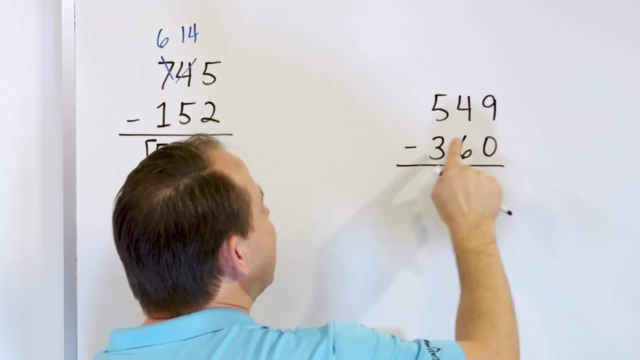 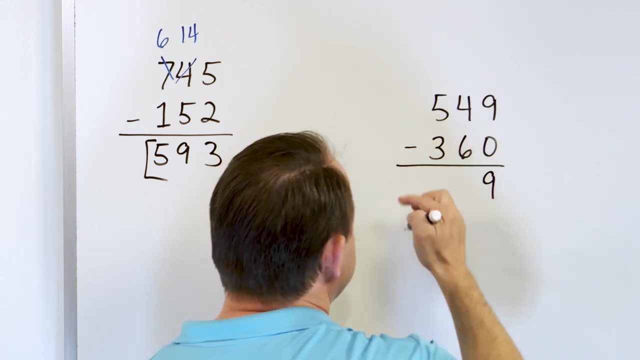 we have 549, and we'll subtract from that 360.. So we go in the right-hand column: What is 9 minus 0?? We start with 9.. We take away nothing, so we are left with 9.. Then we go 4 minus 6, but we 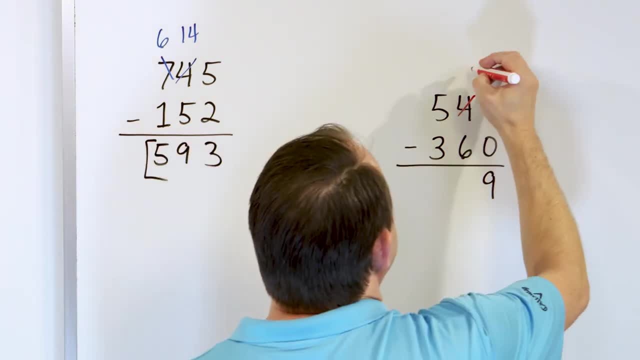 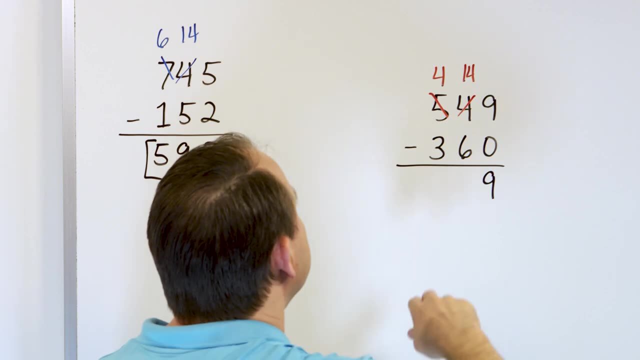 can't do that because 4 is not big enough. So we change that 4 into a 14.. How do we do that? We change the 5 next door into a 4.. We borrow from the next door What is 14 minus 6?? 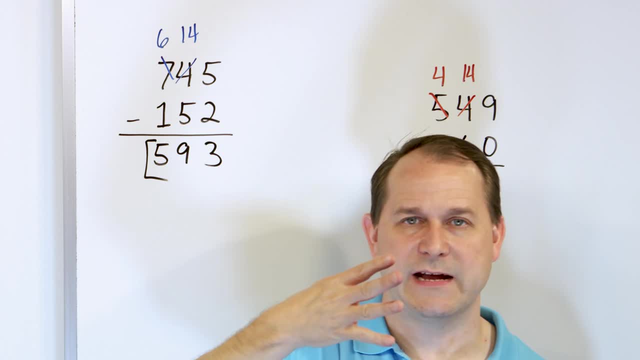 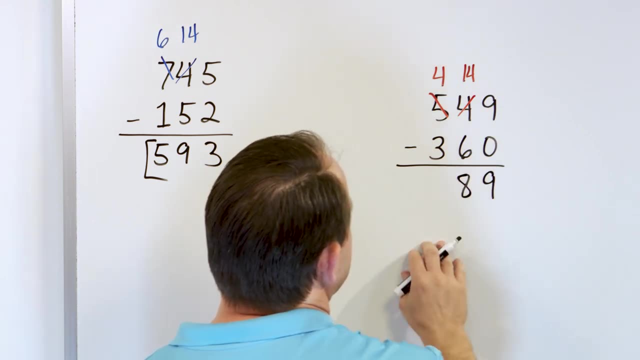 Start with 14 and go down 13,, 12,, 11,, 10,, 9,, 8.. And we land on 8.. So 14 minus 6 is 8, and so 8 goes in this column. Now, what is 4 minus 3?? You probably know the answer, but start with. 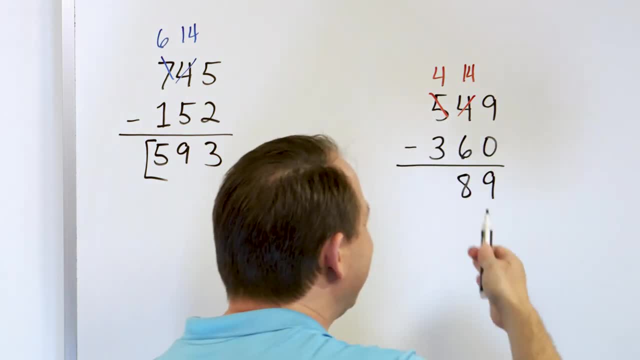 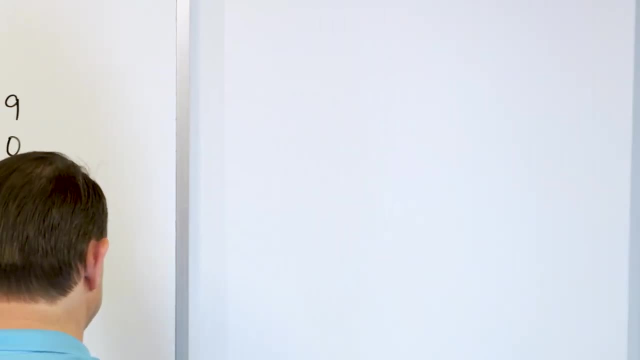 4.. Go down 3,, 2,, 1.. We land on the number 1.. Makes sense. Start with 4.. Subtract 3.. You're going to have 1 left. So the answer is 189.. All right, great, Let's continue on here. What if we? 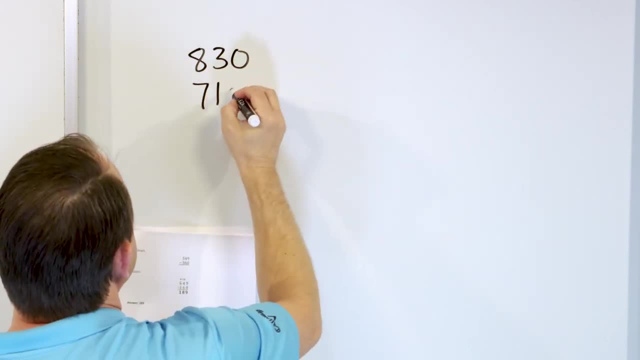 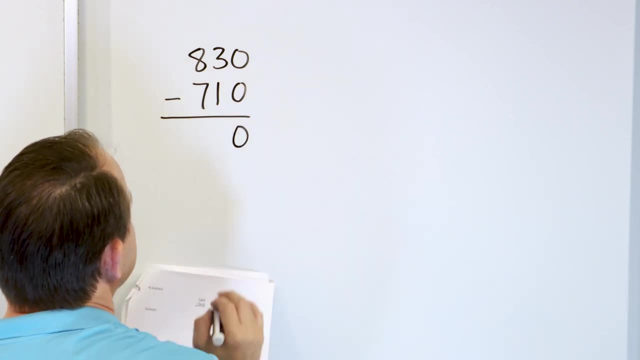 have 830? And we'll subtract from that 710.. Now in the right column, 0 minus 0.. You start with nothing, You take away nothing, You still have nothing. 0 minus 0 is 0.. 3 minus 1 is very easy. Start with 3.. Go. 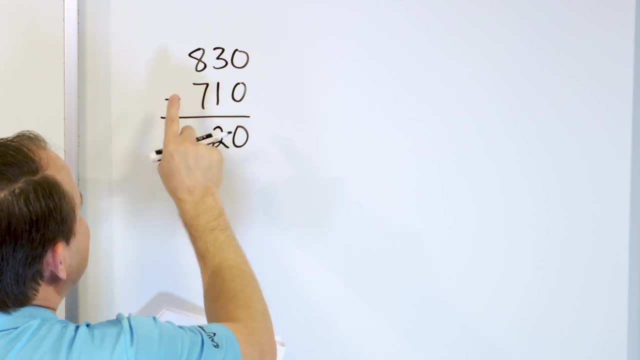 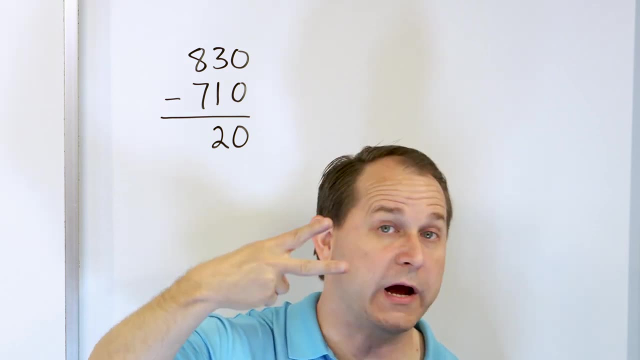 down by 1, and you get to 2.. 8 minus 7 is also easy. You probably know the answer, but if you don't remember, start with 8.. Go down 7,, 6,, 5,, 4,, 3,, 2,, 1.. So 8 minus 7 is 1.. Makes sense, You? 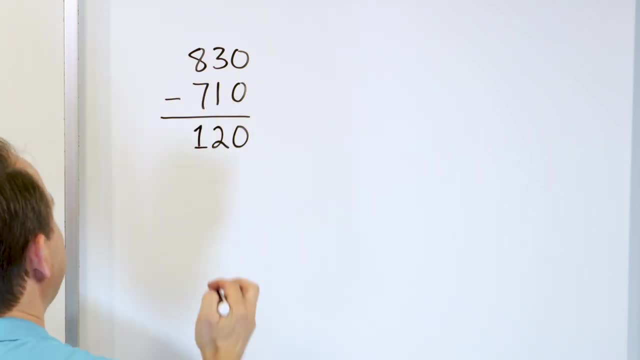 start with 8, and you take away 7. You're going to have 1 left, So the answer is 120.. We didn't have to borrow anywhere in that problem, because all the numbers on the top were bigger than the numbers on the bottom, or equal. 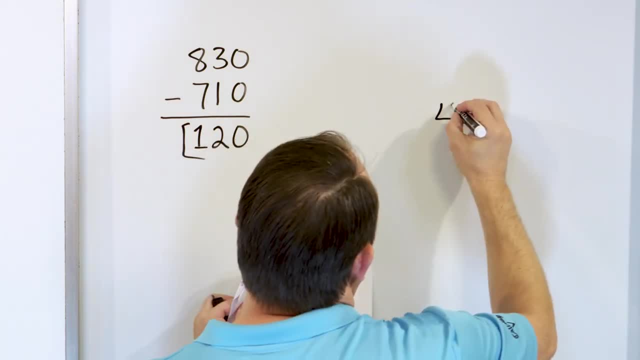 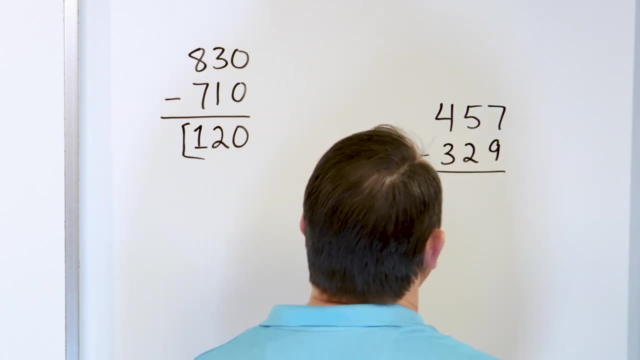 to in the case of the 0. Now we have 457, and we'll subtract from that 329.. All right, so what do we do next? We look in the right column, 7 minus 9.. The problem is 7 is not big enough to. 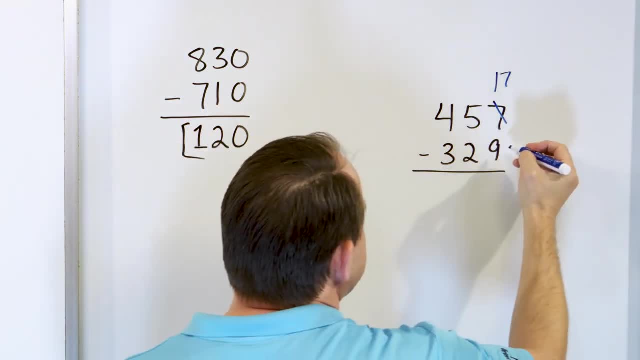 take away 9,. so we change that. We take away 9, and we subtract from that 329.. So we have 7 into a 17.. In order to do that, the 5 becomes a 4.. So we have 17 minus 9.. Start with 17 and go. 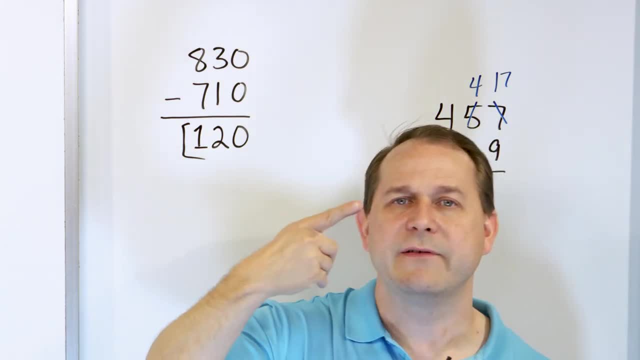 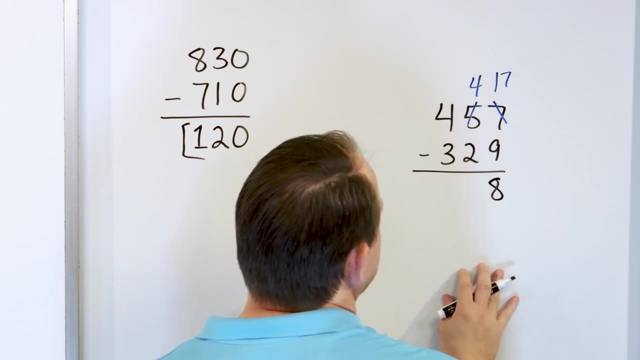 down 16,, 15,, 14,, 13,, 12,, 11,, 10,, 9,, 8.. So we say that 17 minus 9 is actually 8, and so 8 goes in this column Here: 4 minus 2.. You all know that 2 plus 2 is 4.. So if we start at 4 and we take 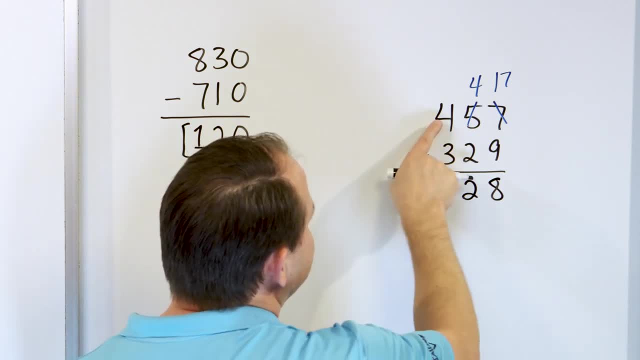 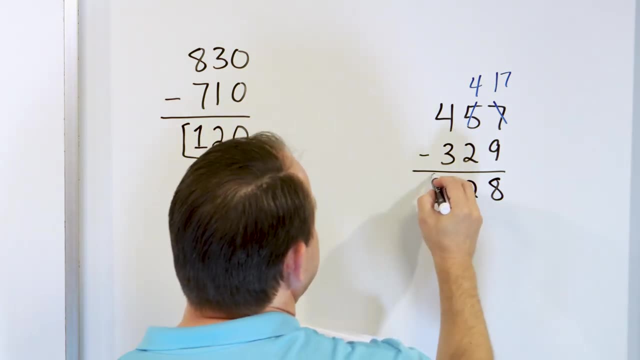 away 2,. what do we get? 2.. Same thing here: 4 minus 3.. Start with 4, and we subtract from that 329.. Start with 4,, take away 3.. The answer we get and we have left is 1.. So we have 128.. That's the. 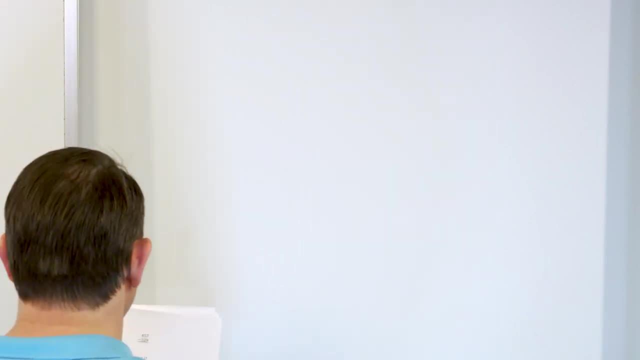 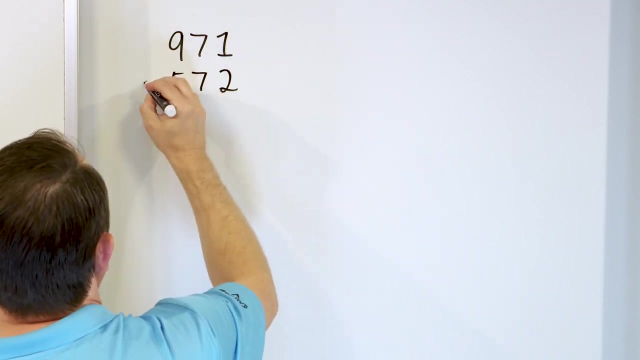 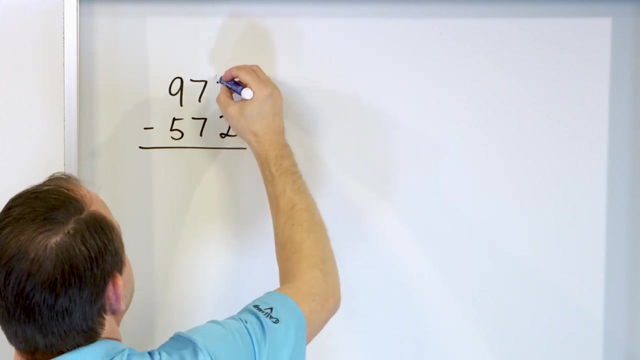 final answer: Okay. next we have 971 minus 572.. Same process: Start with 1 and subtract 2, but you can't do it because 1 is not big enough, So the 1 will become a 11.. How do we do that We? 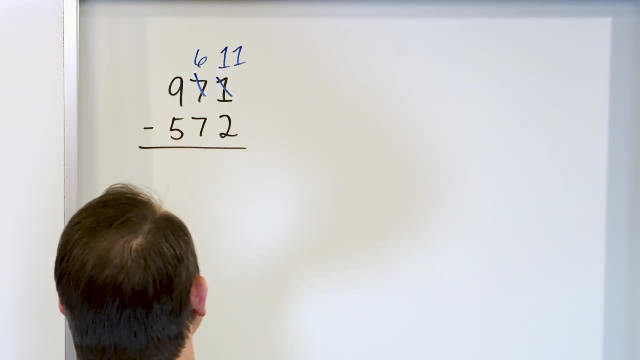 borrow from next door: The 7 becomes a 6. So we subtract from that 329, and we subtract from that 6.. Now we say: what is 11 minus 2?? Start at 11,, go down 10,, 9. And we land on 9.. So 11 minus 2 is: 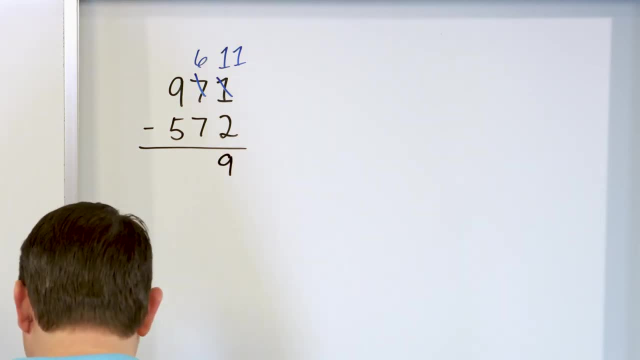 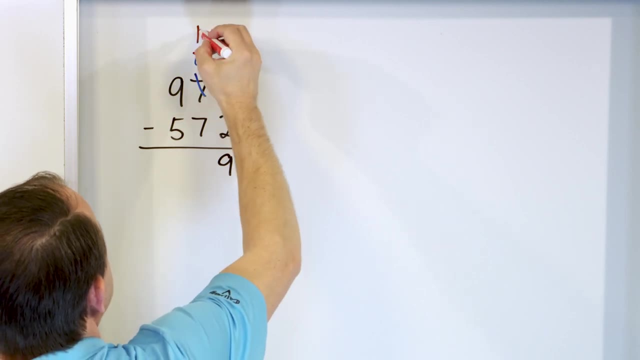 9, and so 9 goes right here. Now we go to the next door neighbor and say what is 6 minus 7?? But that's not big enough. We have to have something larger. so we change the 6 into a 16.. And to do that 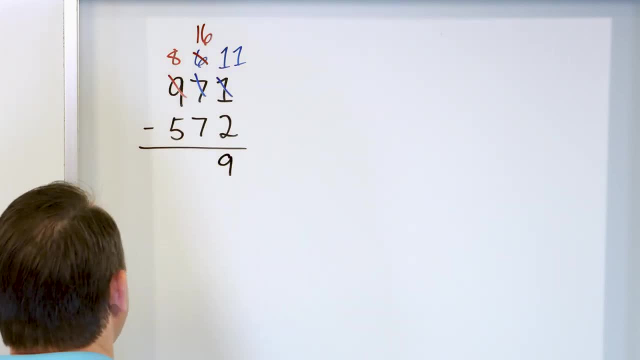 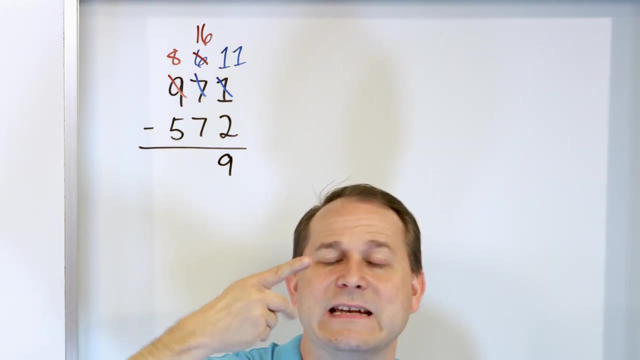 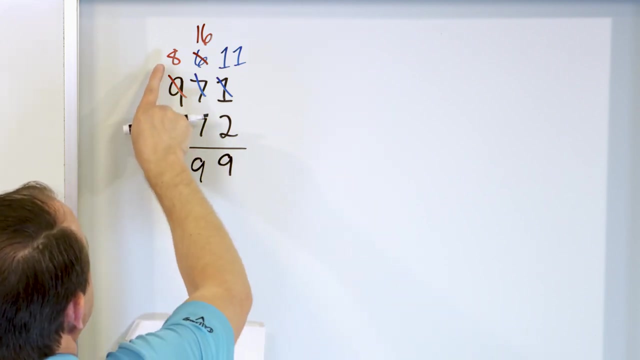 the 9 must then become an 8.. So then, what is 16 minus 7?? Start with 16 and go down 15,, 14,, 13,, 11,, 10,, 9.. So 16 minus 7 is 9.. All right, next we go 8 minus 5.. Start with 8 in your mind, Go. 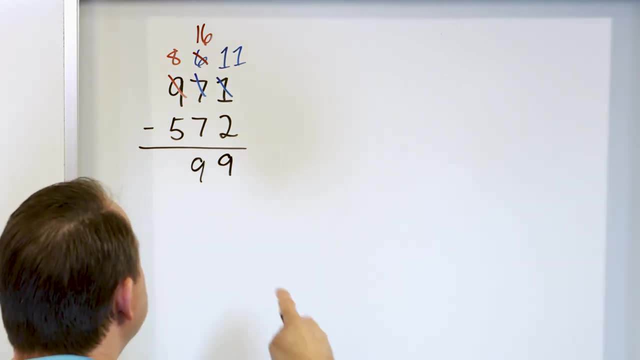 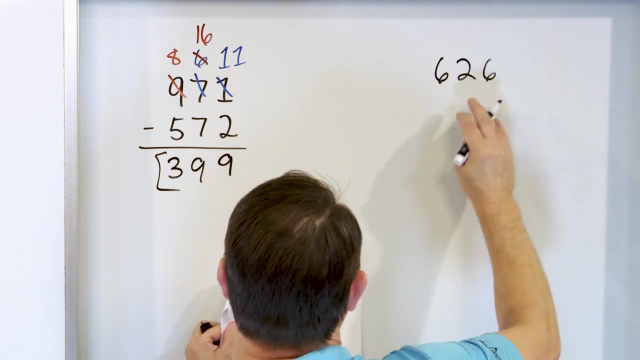 down 7, 6, 5,, 4, 3.. So 8 minus 5 is 3, and the answer we get is 399.. And so 971 minus 572 is 399.. Great, just a few more problems. What if we have 626, and we'll subtract from that. 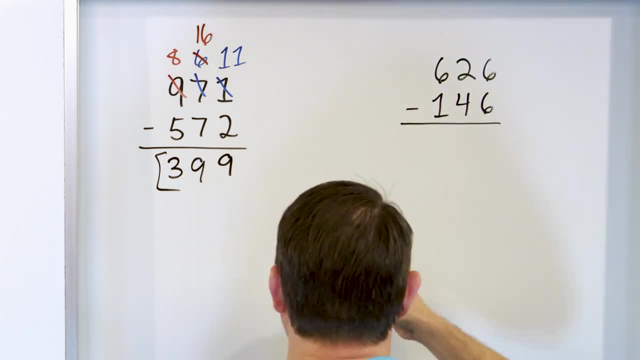 146?? Okay, in the right-hand column, what happens when we start with 6 and we take 6 away? Well then, we don't have anything left. 6 minus 6 is 0.. Now we go over to 2.. 2 minus 4.. Can't really do. 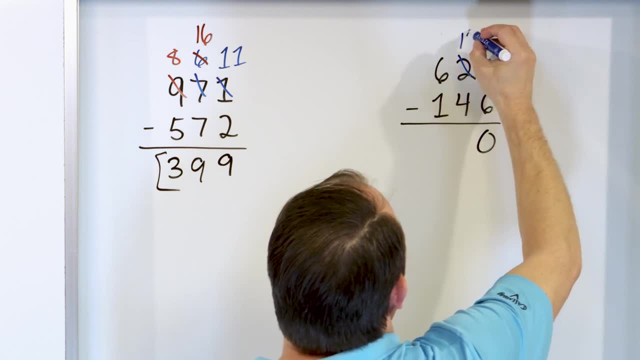 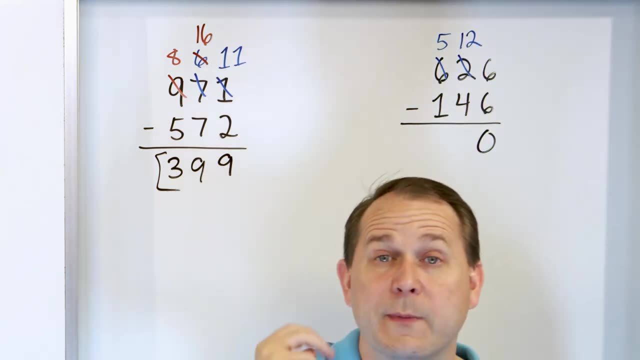 that because 2 is not big enough, So we change this 2 into a 12.. In order to do that, the 6 must become a 5.. 12 minus 4.. Start with 12 in your mind, Go down 11,, 10,, 9,, 8.. And so the answer we land. 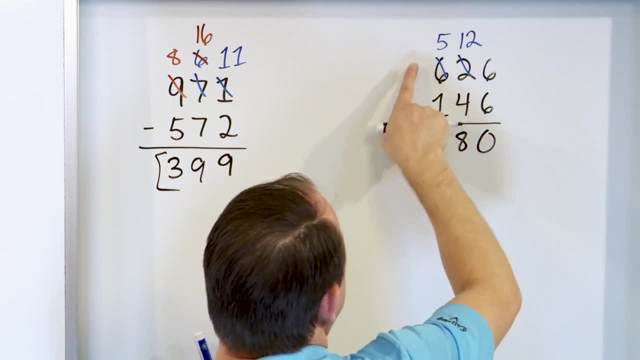 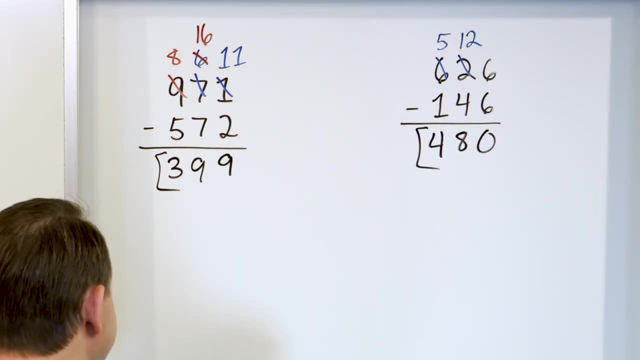 is 8.. Now we go to this column 5 minus 1. You just start with 5.. You go down by 1.. You get to 4.. And the answer is 480.. All right, only two more problems. What if we have 721, and we subtract? 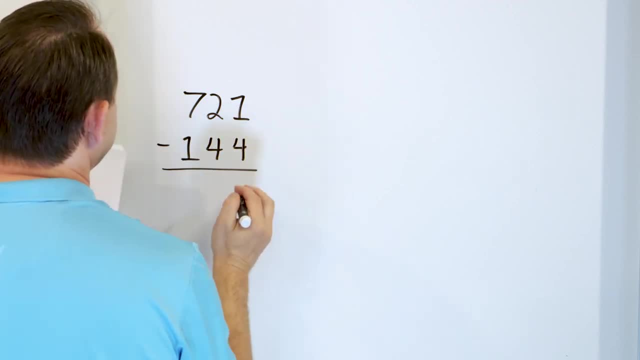 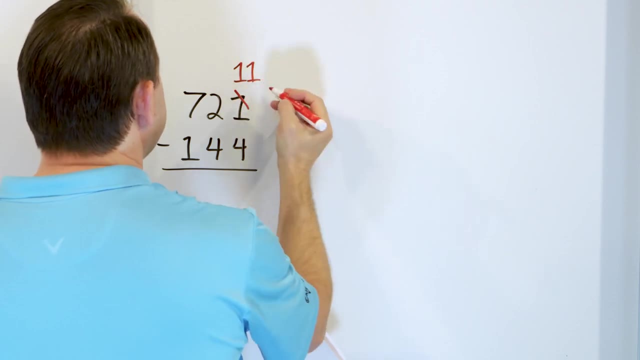 from that 144?? So we start in the right-hand column. We say: what is 1 minus 4?? We can't do that, So we change the 1 into an 11. In order to do that, the 2 must then become a 1.. 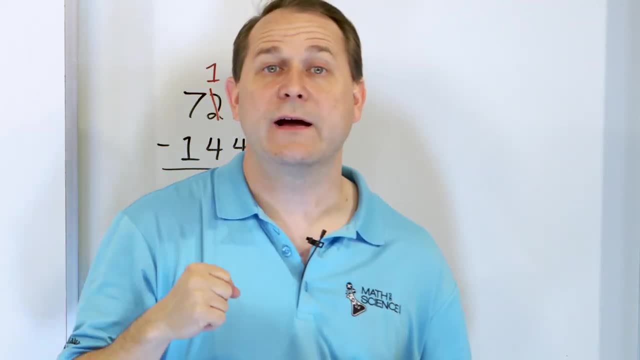 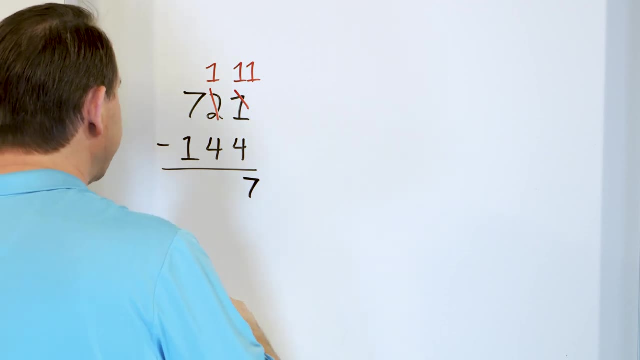 So what is 11 minus 4?? Start with 11.. Go down 10,, 9,, 8,, 7. And we land on 7.. So 7 goes right here. Next we go to the next column. Let's say what is 1 minus 4?? We can't do that, because 1 is. 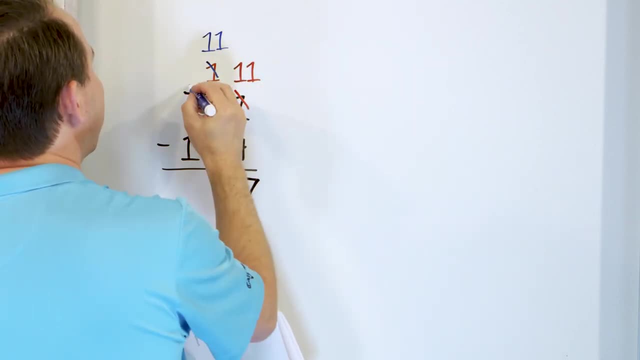 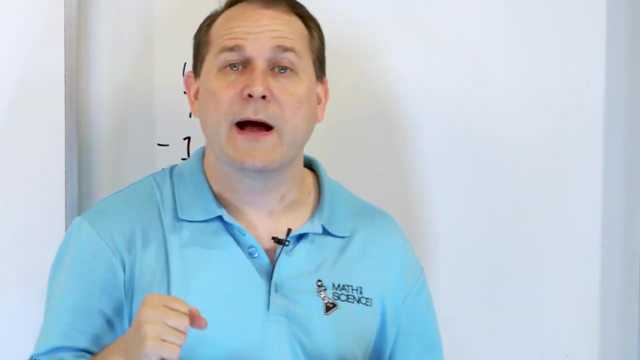 not big enough, So the 1 becomes an 11.. In order to do that, we have to borrow and make the 7 a 6.. So then we say: what is 11 minus 4?? Start with 11 in your mind, Go down 10,, 9,, 8,, 7.. And so the 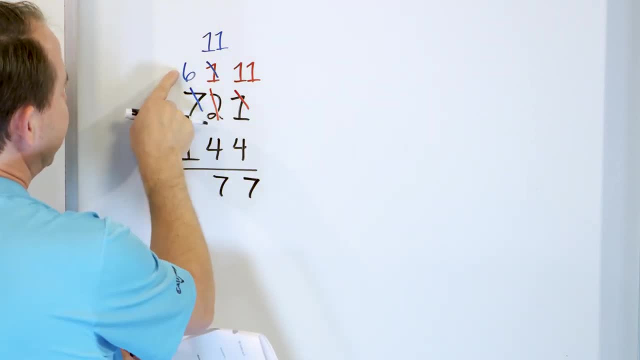 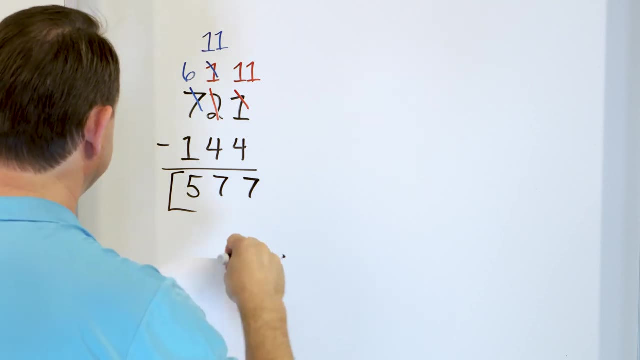 answer is 7.. 11 minus 4 is 7.. Now we say: what is 6 minus 1?? We start at 6, and we go down by 1 to get to 5.. So we get 577 for the answer. OK, only one more problem left. We have 863,. 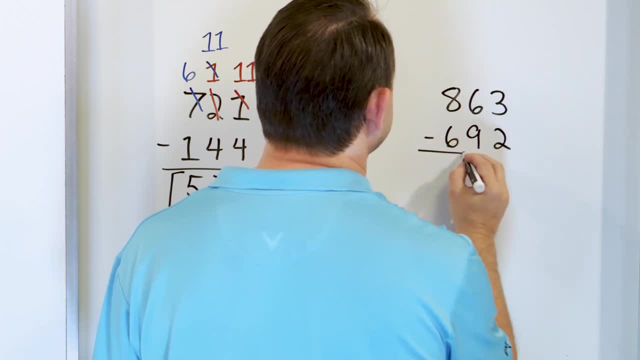 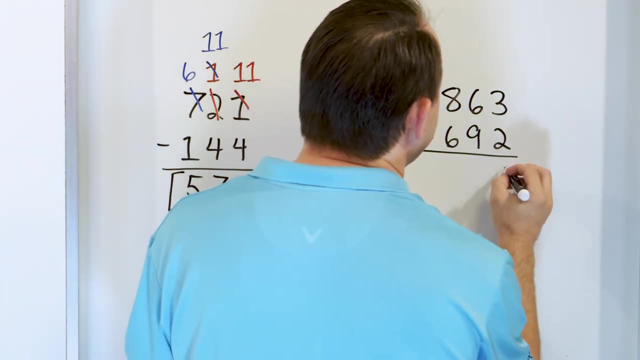 and we'll subtract from that 692.. All right, so we go over to the right and we say: what is 3 minus 2?? Well, if we start with 3, and we take 2 away, the answer that we have is 1 left. 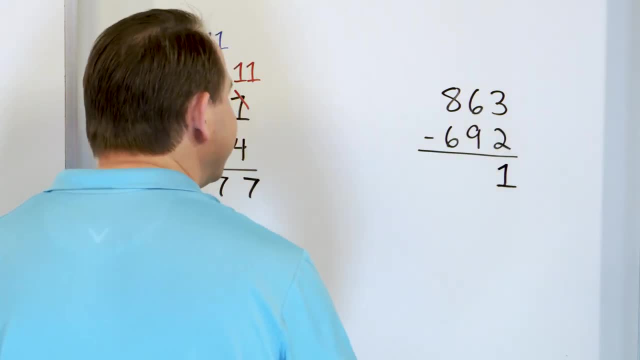 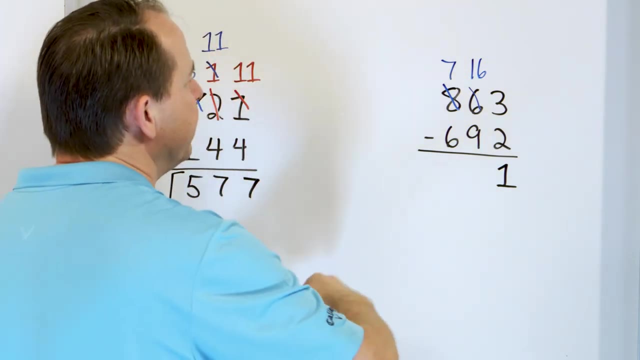 Then we go to this column 6 minus 9.. Can't really do that, because 6 is not large enough, So we'll make it 16 here. In order to do that, we have to borrow and make the 8 into a 7.. 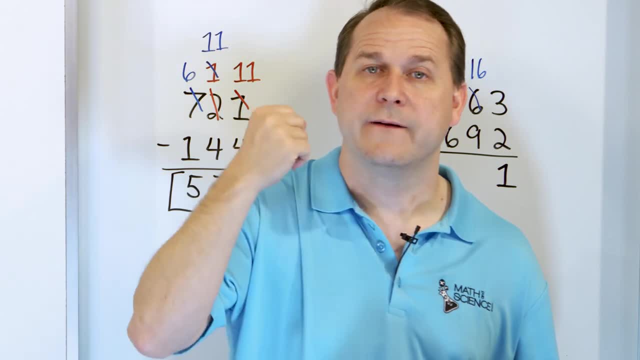 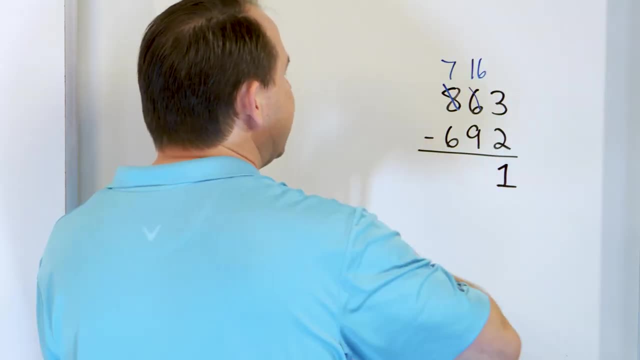 16 minus 9.. Start with 16, and go down 15,, 14,, 13,, 12,, 11,, 10,, 9,, 8,, 7.. So 16 minus 9 is 7,. 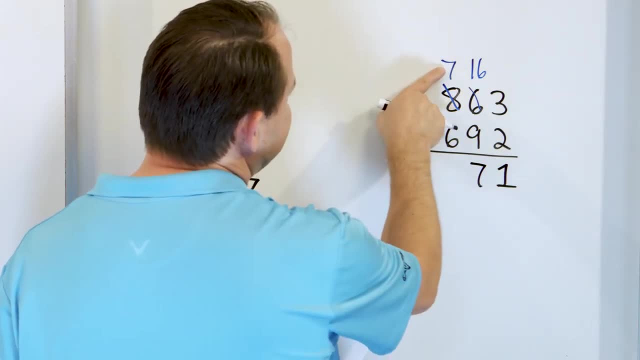 and so 7 goes in this column right here. Next, what is 7 minus 6?? If you start with 7, and you take away 6,, how many do you get? 7 minus 6 is 7.. So 7 goes in this column right here. 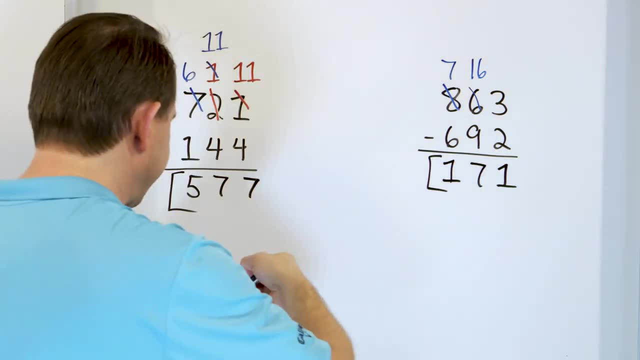 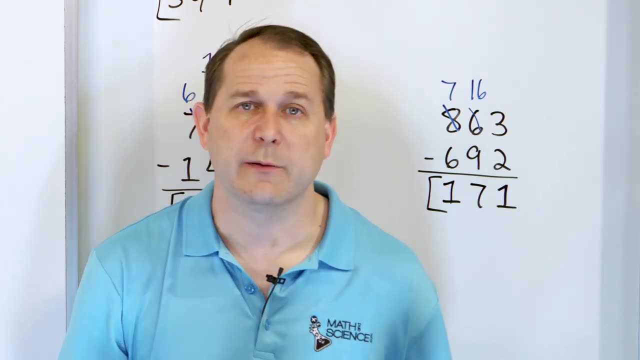 You only have 1 left, So you have 171.. So in this lesson we have gotten a lot of practice with subtracting three-digit numbers. You can see, sometimes you have to borrow, sometimes you don't have to borrow, also called regrouping. Sometimes when you regroup you only have to do.